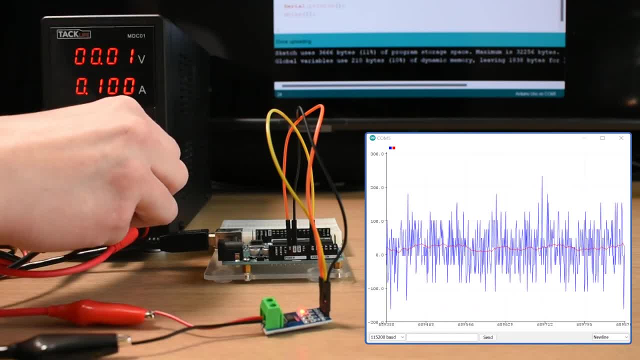 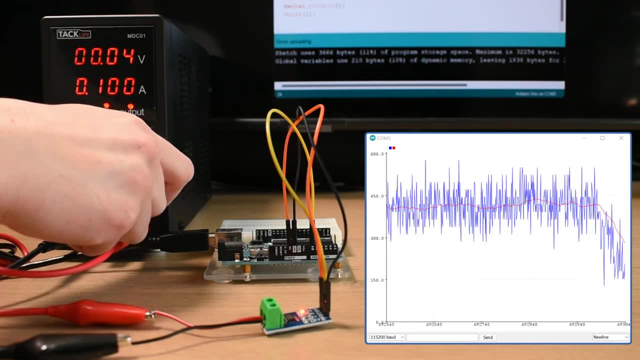 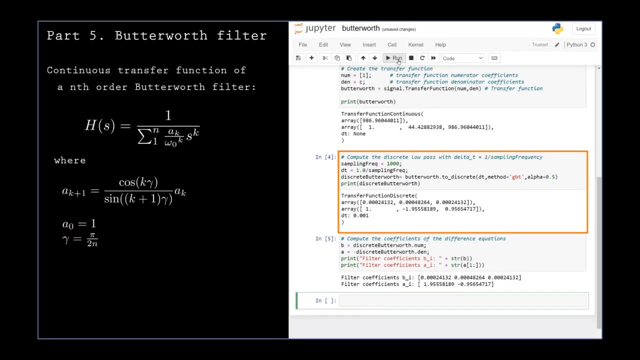 This sturdy signal is starting to look much cleaner. But of course I started to wonder: Could tweaking the filter further improve the current readings? In my last implementation, I had to derive the coefficients in Python and then copy and paste them into the Arduino code. Too much work, right? So here's what I did. 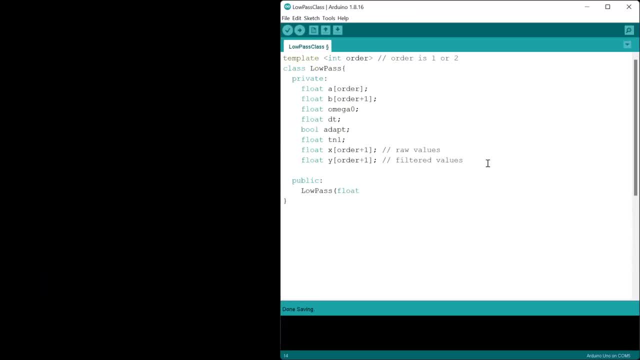 I created a brand new but still super simple digital low-pass filter that allows you to adjust the cutoff frequency and automatically computes the coefficients inside the Arduino code- No Python required. I'm calling it Arduino Digital Low-Pass Filter 2.0.. Here's how you. 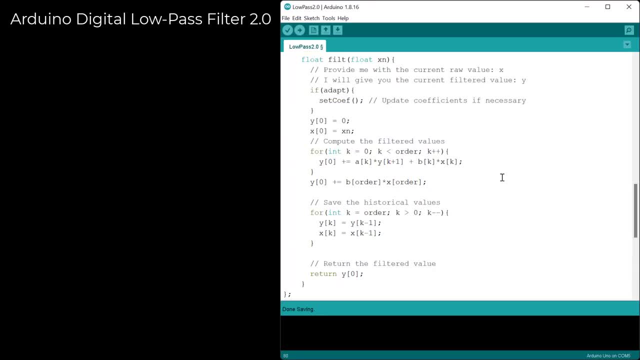 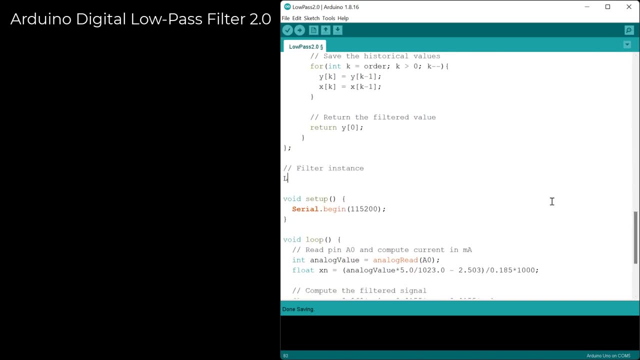 can use it. Copy the low-pass class to the top of your Arduino code. Then create one instance of the class. for each signal you want to filter, Four parameters are required by the constructor. I've only implemented a first-order filter and a second-order Butterworth, so the choice 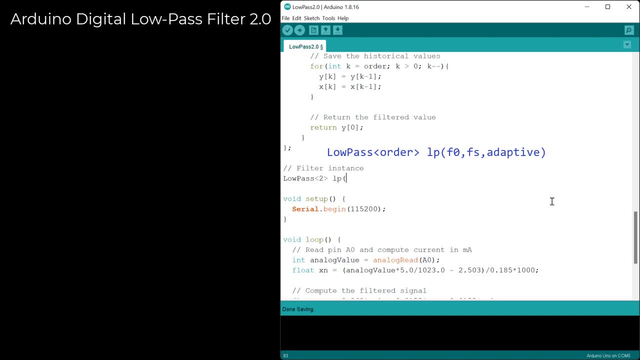 is easy. One or two. Second, set the cutoff frequency in Hertz. Third, set the sampling frequency. This is an issue because we don't usually know the sampling frequency on an Arduino, largely because it changes depending on the code that is running in the loop function. I'll guess. 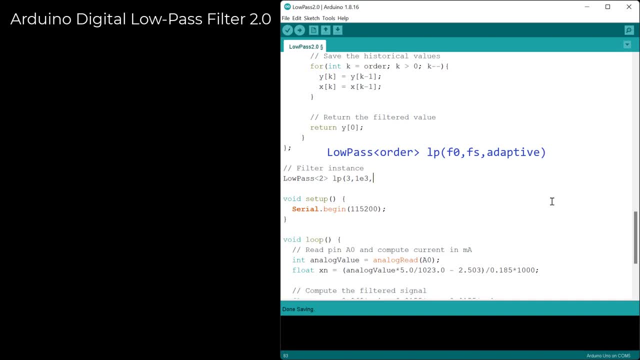 1 kHz. but I know it's wrong. This is why I added the fourth parameter: A Boolean flag. When true, this flag causes the sampling frequency to be computed from the duration of the consecutive steps of the loop function. Now to apply the filter, just call the Filt method with the raw signal as the input. 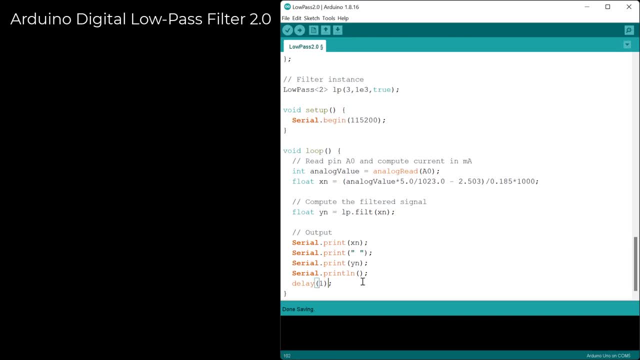 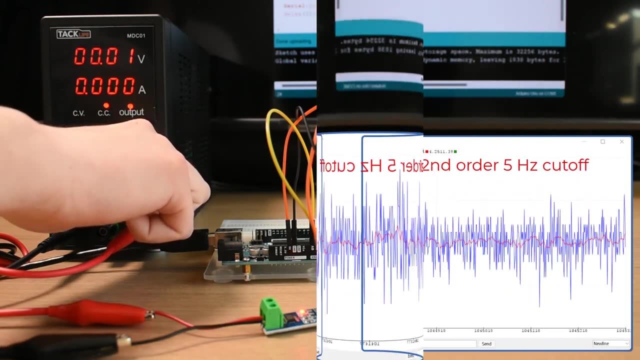 The output will be the filtered signal. Here's the first-order result. Increasing the order to 2 improves the result. Here's the first-order result. Increasing the order to 2 improves the result. Increasing the order to 2 improves the result. 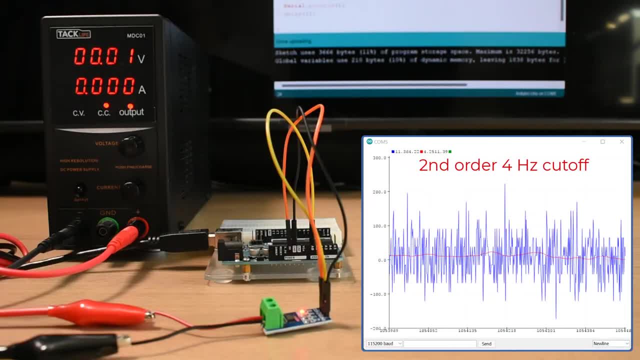 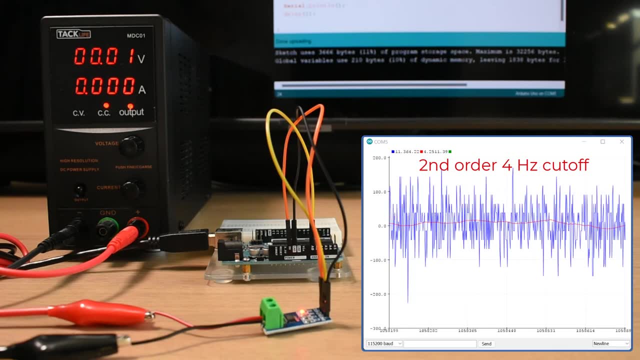 But adds more delay For this signal. I'm liking the second-order filter with a 4 Hz cutoff. If you have dirty signals too, you can find my code to clean them up linked in the comments below.